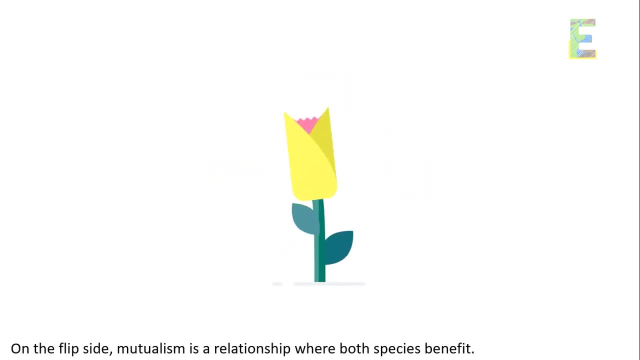 Neutralism. On the flip side, mutualism is a relationship where both species benefit. It's a win-win scenario. For example, the relationship between bees and flowers, where bees pollinate flowers while obtaining nectar, is a classic example of mutualism- Commensalism- Commensalism is 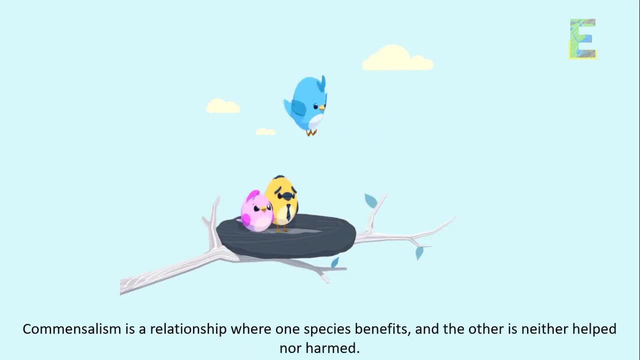 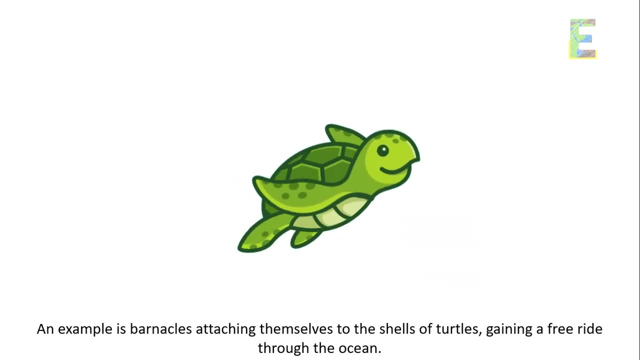 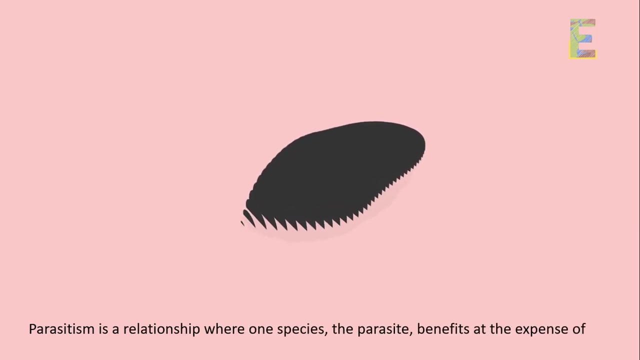 a relationship where one species benefits and the other is neither help nor harm. An example is barnacles attaching themselves to the shells of turtles Gaining a free ride through nature, The ocean- Parasitism. Parasitism is a relationship where one species 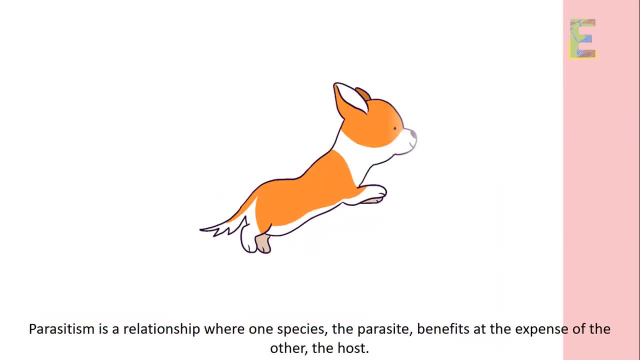 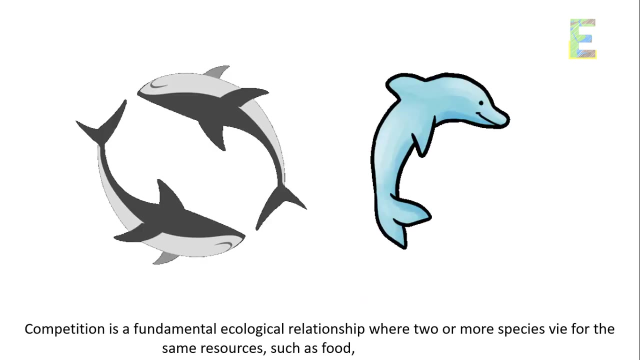 the parasite benefits at the expense of the other. the host Parasites can be external, like ticks, or internal, like tapeworms, and they often cause harm to the host. Competition Competition is a fundamental ecological relationship where two or more 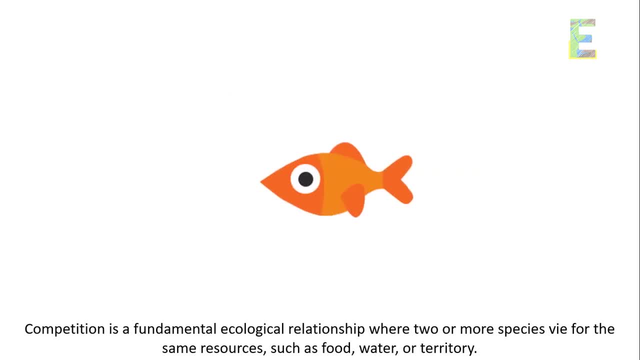 species vie for the same resources, such as food, water or territory. This competition can be intense and shape the distribution and abundance of species. Symbiotic relationships: some ecological relationships are more specialized and long-term, leading to symbiotic relationships. 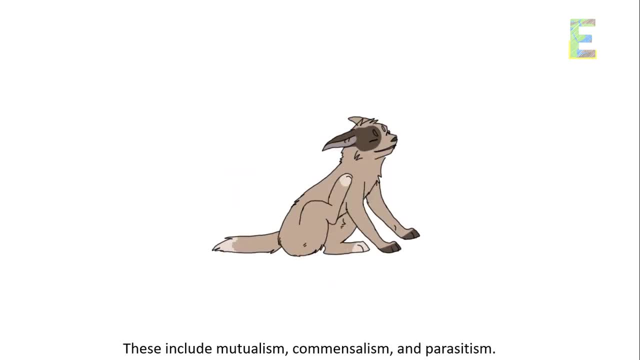 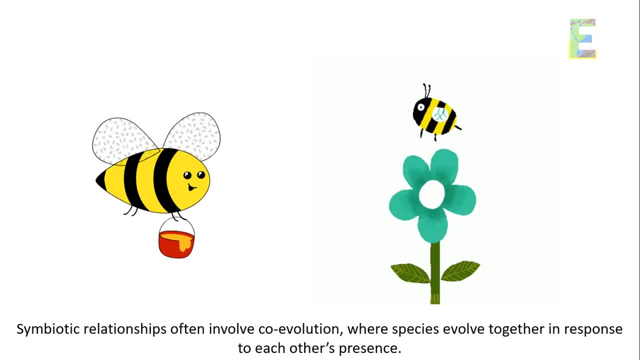 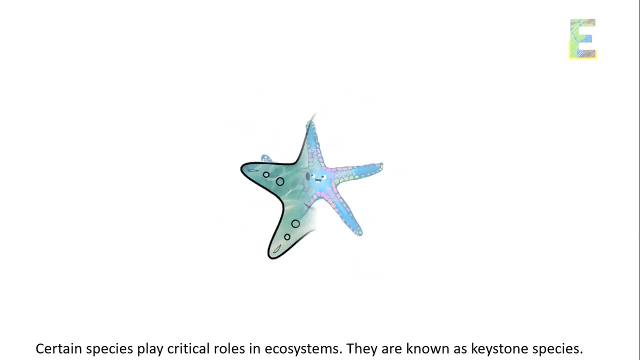 These include mutualism, commensalism and parasitism. Symbiotic relationships often involve co-evolution, where species evolve together in response to each other's presence. Keystone species: certain species play critical roles in ecosystems. They are known as keystone species. 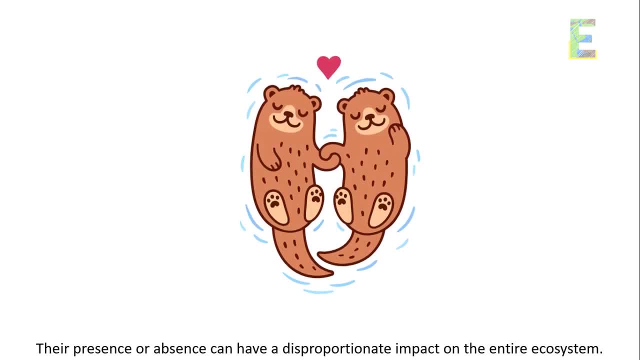 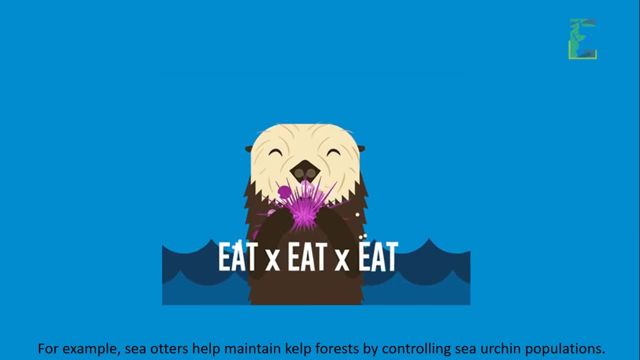 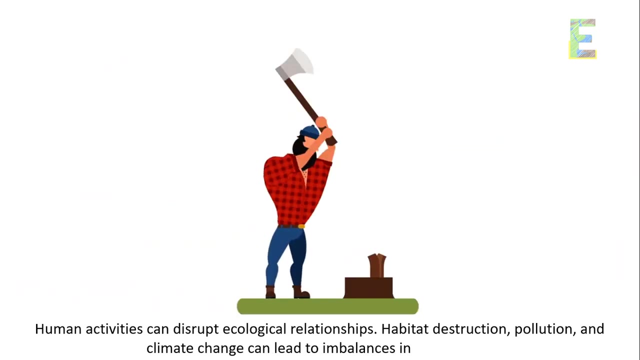 Their presence or absence can have a disproportionate impact on the entire ecosystem. For example, sea otters help maintain kelp forests by controlling sea urchin populations. Human impact- human activities can disrupt ecological relationships, Habitat destruction, pollution and climate change. 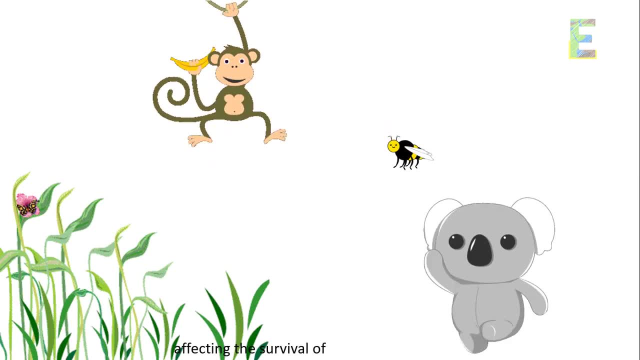 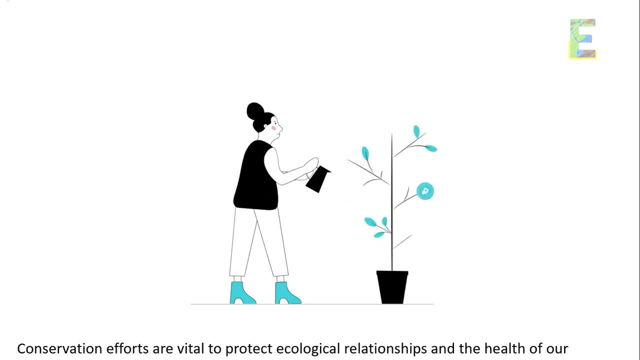 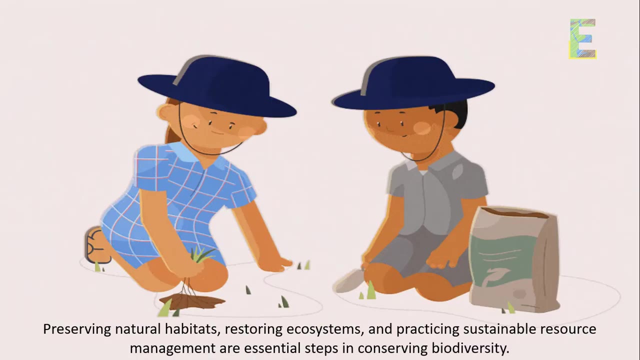 can lead to imbalances in ecosystems, affecting the survival of species and biodiversity Conservation. conservation efforts are vital to protect ecological relationships and the health of our planet. Preserving natural habitats, restoring ecosystems and practicing sustainable resource management are essential steps in conserving biodiversity.